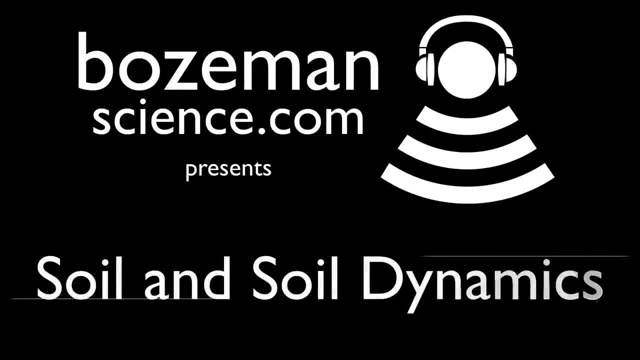 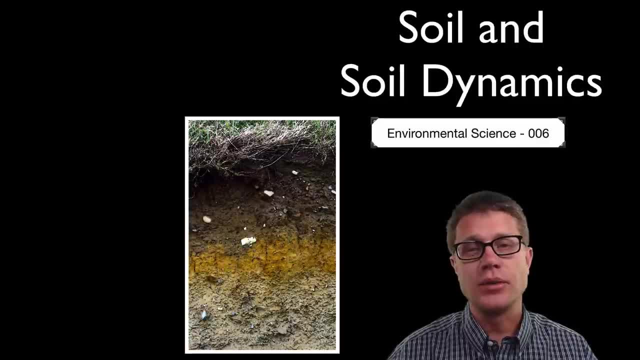 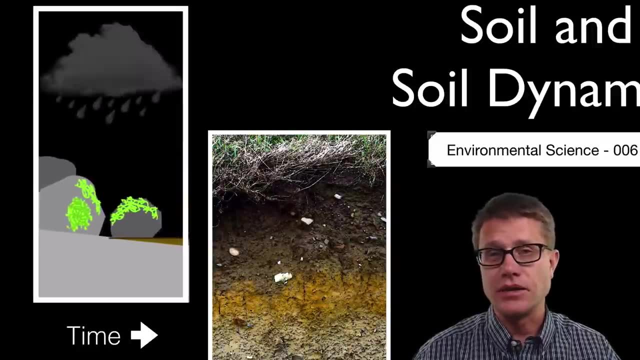 Hi, It is Mr Andersen and this is environmental science, video 6. It is on soils. Soils are incredibly important. It is where we grow our food, But they take a long time to form. We start with regular rock And then, over time, what we have is weathering. We have physical 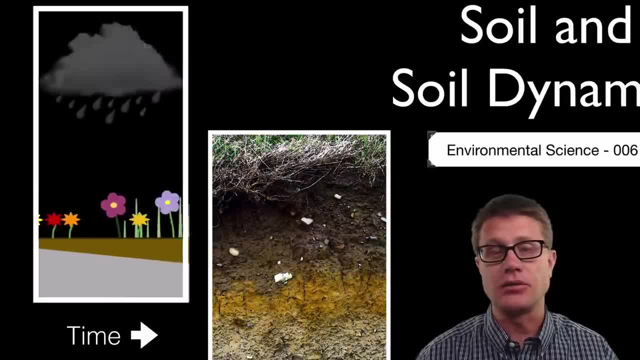 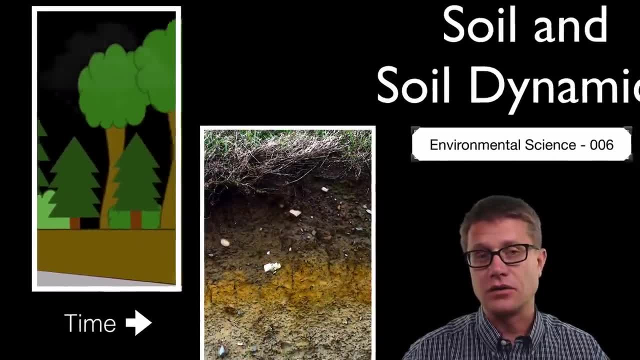 weathering, where we break the rock down into smaller particles. We have chemical reactions or chemical weathering. We have biological weathering as well, And so it takes a long time for us to go from rock to soil- Soil that we can grow our crops in. And the sad 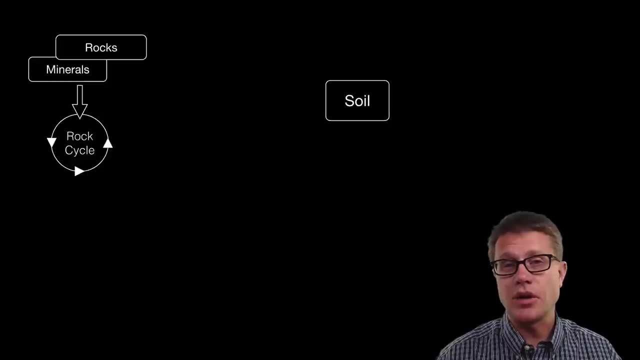 thing is that it can all be lost overnight, And so rocks, remember, are made of minerals which are recycled on our planet using the rock cycle. They can undergo weathering, both physical and chemical, And that produces the particles in the soil. It makes up about half. 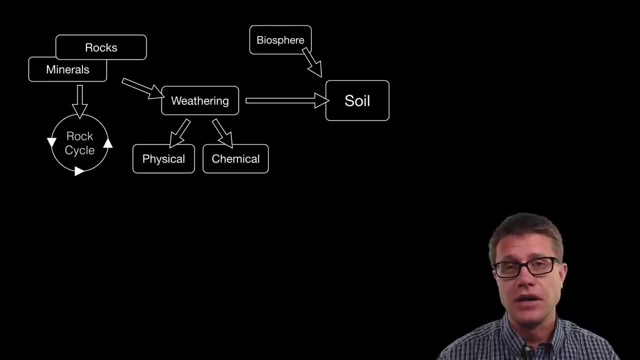 of the soil. We also have the biosphere contributing life. We have the atmosphere and the hydrosphere And also a lot of time, And so all of these contribute to soil. We are going to have lots of different types of soil on our planet. We are going to have soil that is going to 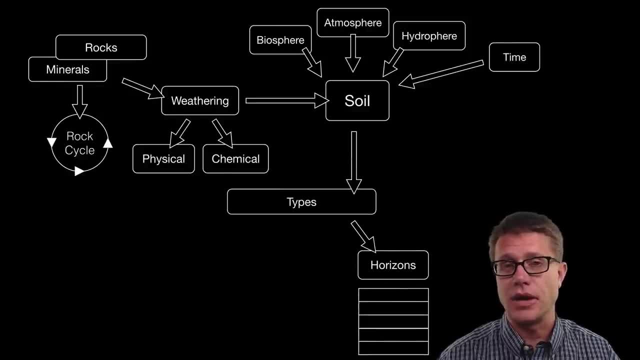 grow on our planet. One way to look at classified soil is to look at the different horizons or the layers in the soil. We could also look at the particle size in the soil Going from large to small. It goes from sand to silt to clay. Now that contributes to the porosity. 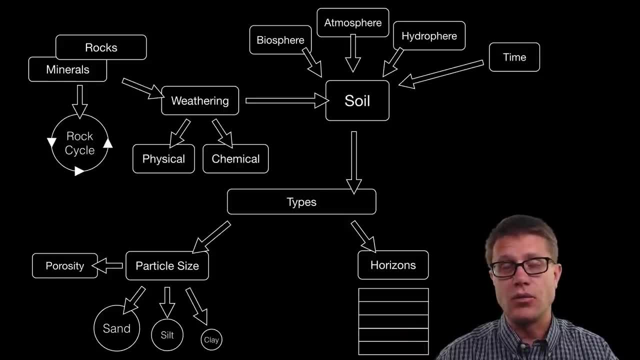 of the soil. How easy is it for the water to get down and bring water and nutrients to the roots of the plant? And then we also have the chemistry of the soil: Where did the parent rock come from? And one of the big things that is important in the chemistry- 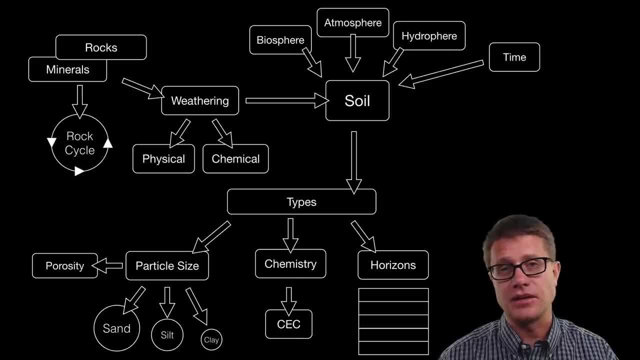 is the CEC or the cation exchange capacity. So the cation exchange capacity of the soil, How easily does that soil deliver important ions to the roots themselves? Conservation is incredibly important with soils. We have soil erosion, where we are physically removing the soil, And then we also have salinization, or salting of the soil, which is contributing. 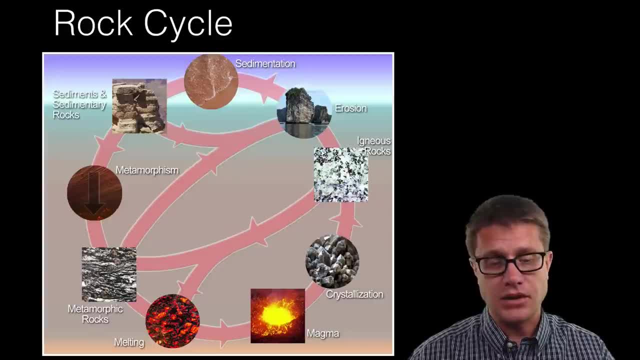 to soil loss. So on our planet, remember, we have a rock cycle where we can move from igneous rock, which are crystallized magma, to sedimentary rock. So we have this weathering, Erosion moves it, And then we have this compaction to form sediment, And then we have this compaction. 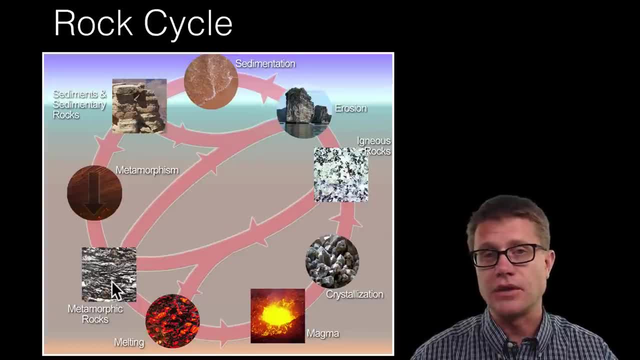 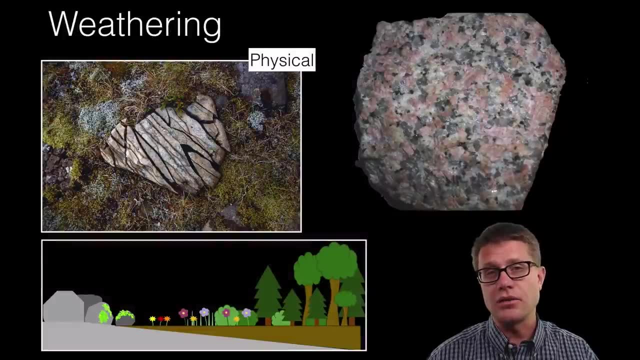 to form sedimentary rocks like sandstone. And then we can have metamorphism, where we are actually putting heat and pressure on that rock to convert it into a metamorphic rock. But it is weathering that contributes to our soils, The first type of weathering. 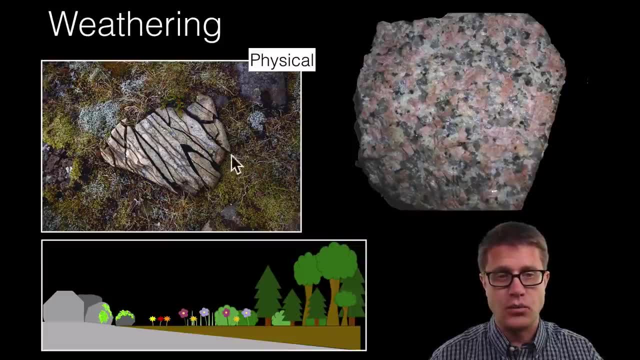 is going to be physical weathering. This is an example of a rock that has been weathered physically. You can see it is just broken apart. So that is water. It could be ice wedging, It could be the roots of a plant, But anything that increases the surface area of the rock. 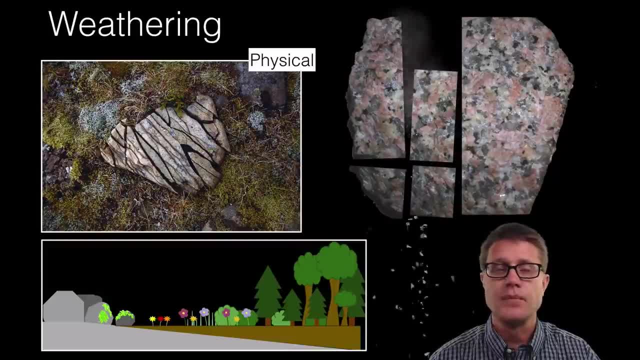 In other words, anything that physically breaks it down. It becomes the rock that gets more water. We have a lot of different kinds of rockplaces. We have rock fibers. We have rock down into smaller bits. that is going to be physical weathering. Now, that is only half. 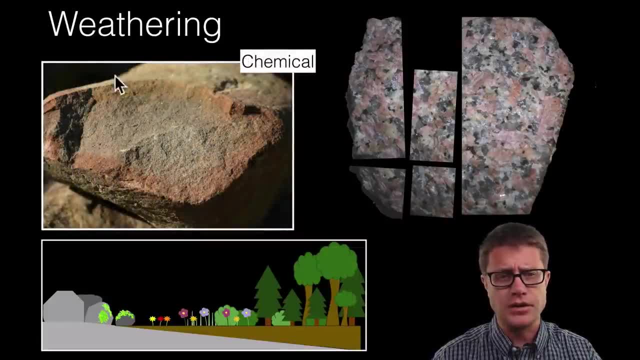 of it. We also have chemical weathering. So on this rock here you can see there is rust or oxidation going on on the outside of that rock And so that chemical reaction breaks down our rock into particles of the soil as well. So if we look at this granite, this 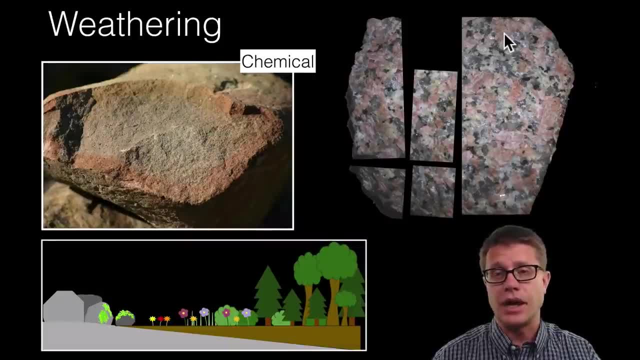 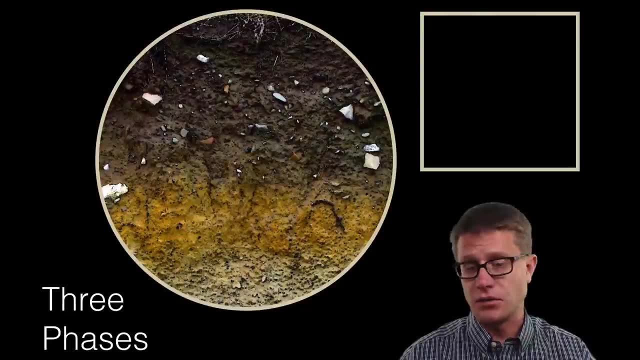 feldspar here- can react with naturally forming acids and form something called clay, And we will talk about the importance of clay in a little bit. Now we can talk about soil being three phases coming together, So we have solid, liquid and gas. If we look at 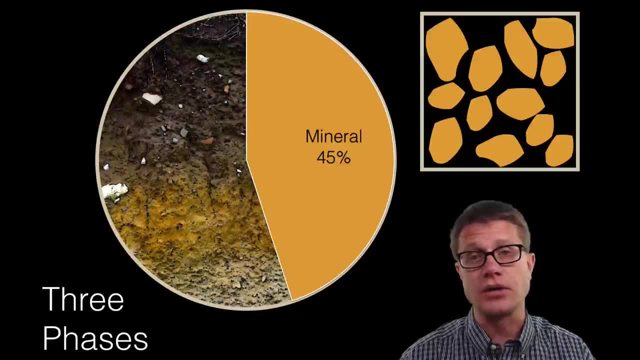 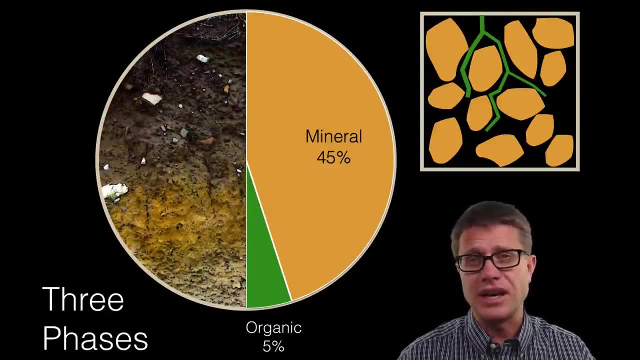 the solid phase we are going to have the minerals of the soil itself, So that was the particles that came from the parent rock. We also have the organic material, So the living material, So roots would be an example- or dead material. We also have the hydrosphere, So the water. 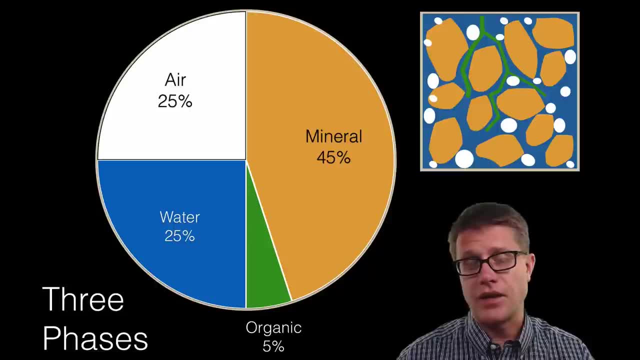 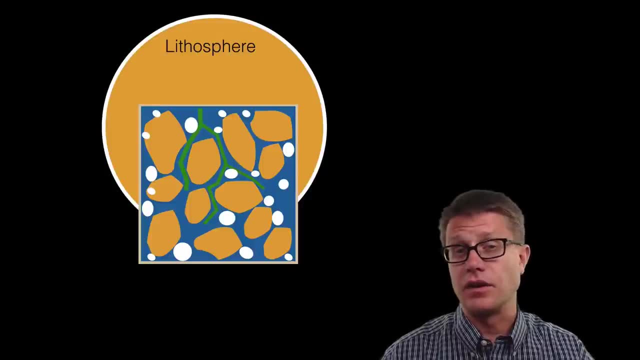 coming together And then we are going to have the air. And so this is the breakdown of how much contributes to the soil. It is going to differ on what soil we have. But if you think about it, what is soil? It is a coming together of the lithosphere, or the 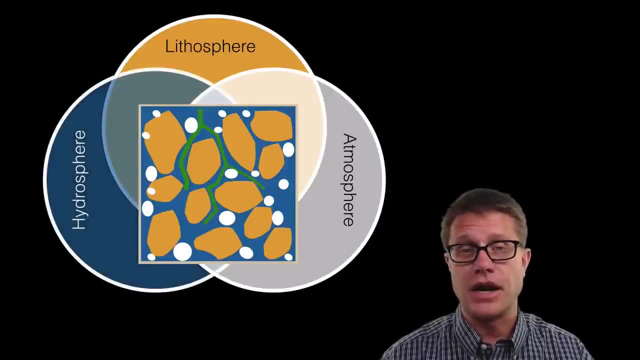 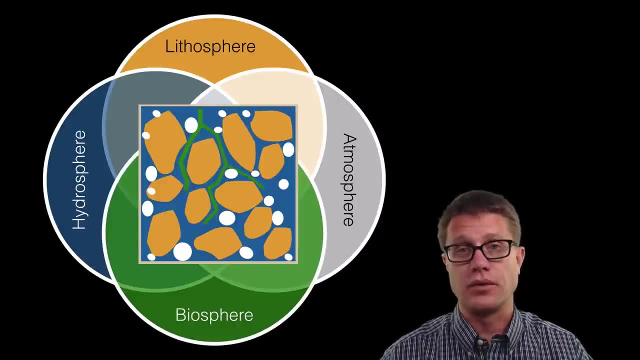 earth, on our planet, It is also the air, or the atmosphere, and the hydrosphere, And then it is where we are headed next in this course. It is the biosphere, the living material, And so that is why soil is important. It is at this interface between all these different 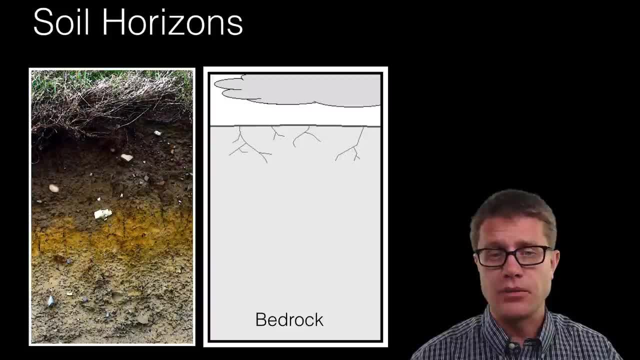 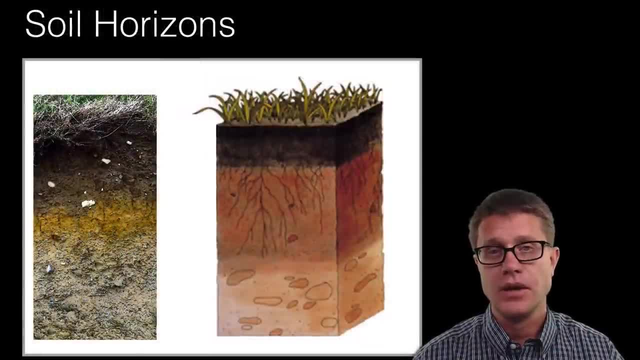 spheres on our planet And if we look at how it is formed, bedrock is broken down, weathered over time and we eventually get what are called the horizons of the soil. We could classify some of the major soil horizons. At the top we are going to have what is called the O-horizon. 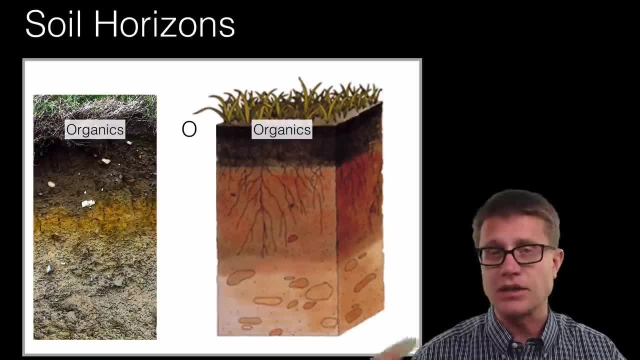 That is going to be the organic. That is going to be where we are going to have a mix of a lot of dead or dying material. Below that, we are going to have the A-horizon. That is going to be our topsoil. That is going 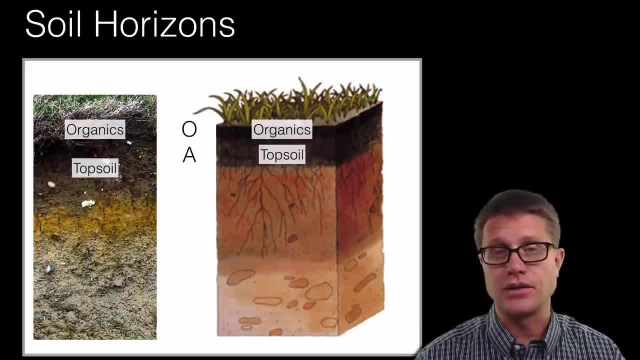 to be a nice mix of minerals and also all the organics from the horizon above. As we go. below that, we are going to have the B-horizon, which is the subsoil. Not a lot of organics found in here. We are still going to have minerals and nutrients that are pushed down. 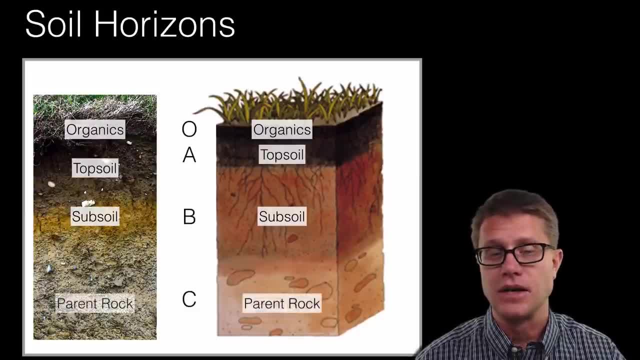 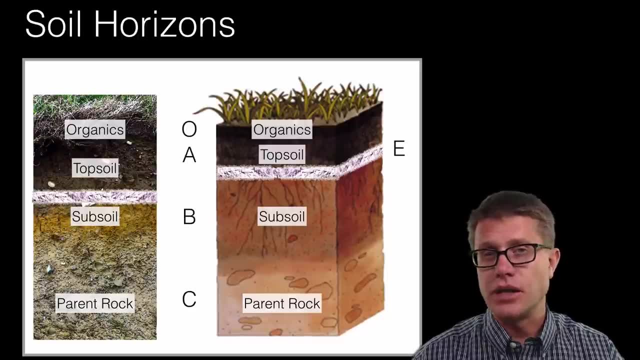 from the soil layers above, And then, finally, we get down to the C-horizon, And that is going to be where we have parent rock. Now, in certain soil horizons we will have different layers of soil. We are going to also have an E-horizon, And so that is alluviation taking place. In other words, we have the movement. 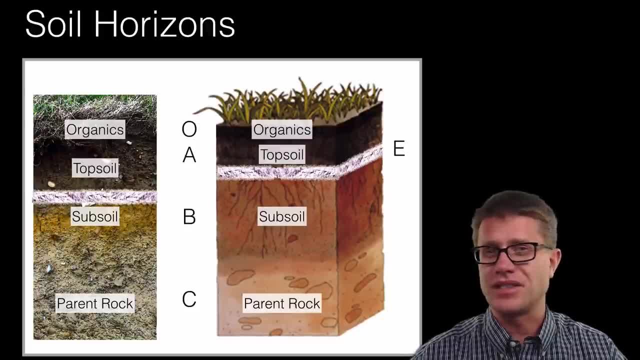 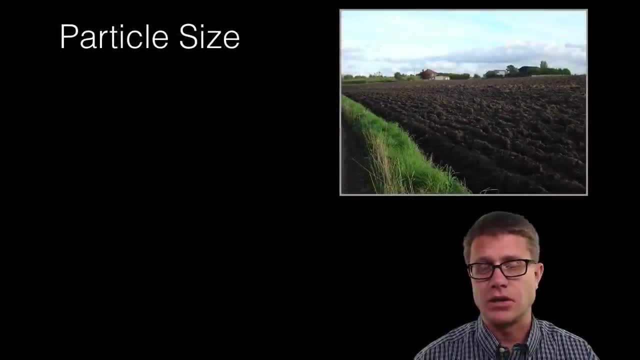 of water down, It is pulling those minerals out And we are just left with sand and silt Kind of this dry layer. Particle size contributes to what type of the soil we are talking about. So this is a loam right here on the right side. So if we look at that soil it is going 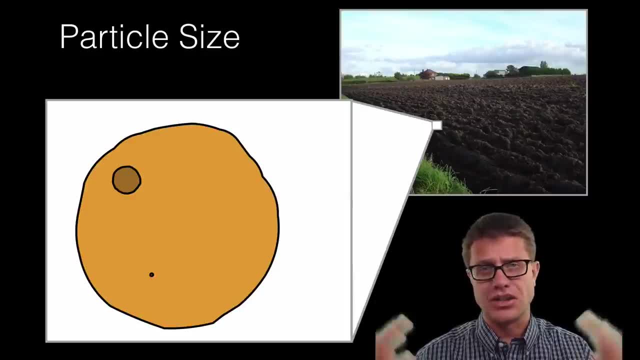 to have varying sizes. We could go from very big like boulder to gravel. But eventually, when we get to the level of the soil, we have got sand. Sand is going to be relatively large in the soil. We then have silt And then finally we have clay. Clay is going to be 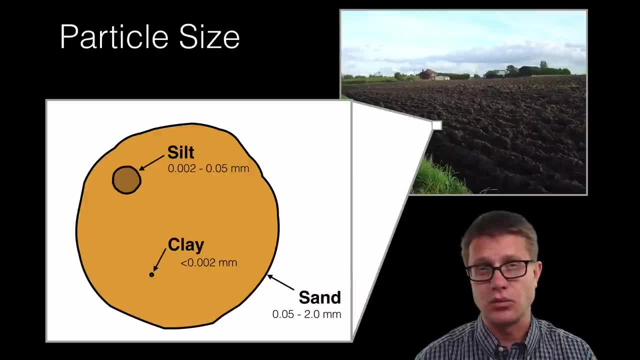 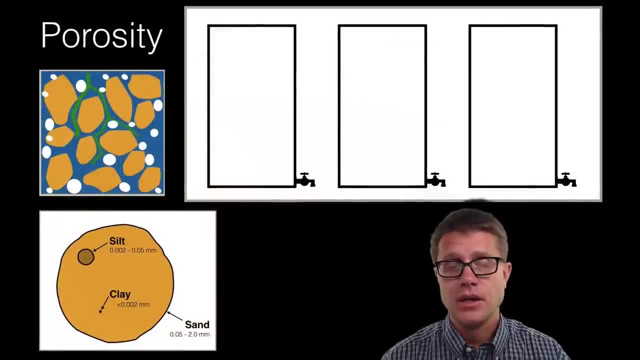 particles that are smaller than two thousandths of a millimeter, So really really fine particles. Now what do those particles contribute to? It is the type of the soil and the porosity of that soil. So let's say we take those three particles and fill up a container with sand. 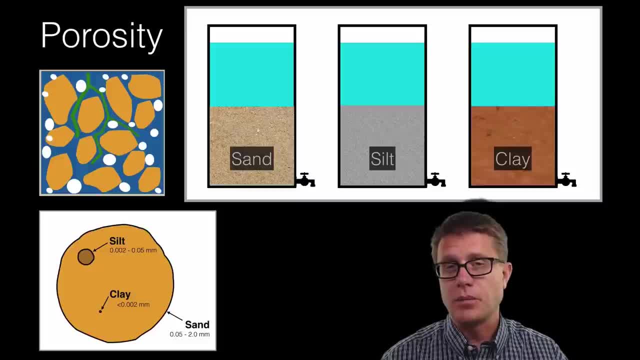 silt and clay and then we fill it up with water. Well, you can imagine what is going to happen In the container that has sand: it is going to drain out, Or we are going to have high porosity And that is going to take hours. So this will be the знаете children's. 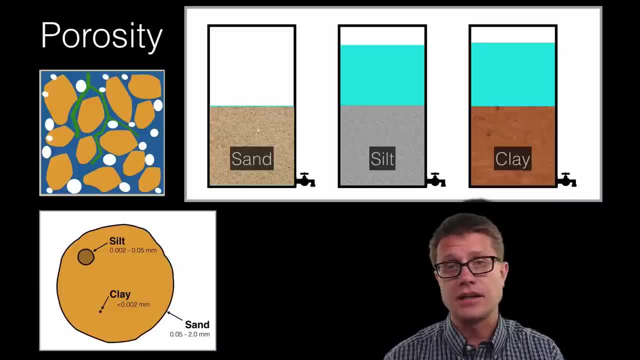 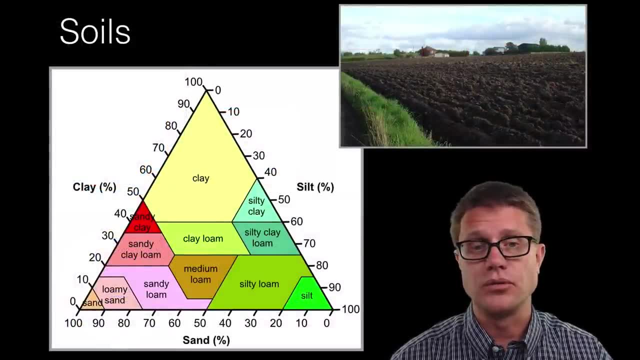 hours. In the silt it is going to take days, And in the clay it is going to take years, And so having a lot of clay can really stifle the movement of water into the pores, where those roots need it. Now we can classify soil based on which of these particles we have. 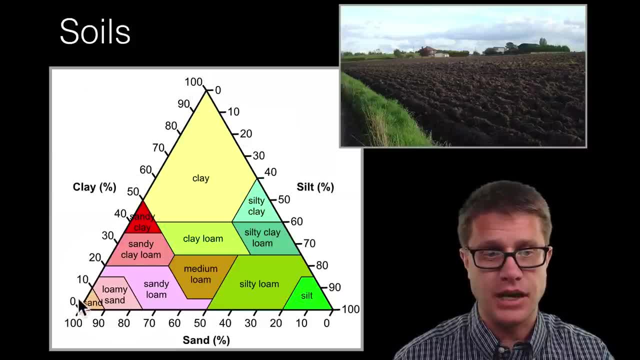 And so this chart takes a second to get used to. So this would be the clay on the left side, from 0% to 100%, And this would be the silt on the right side, and then the sand down below- Remember, in particle size sand is biggest- then silt and then clay, And so you can see. 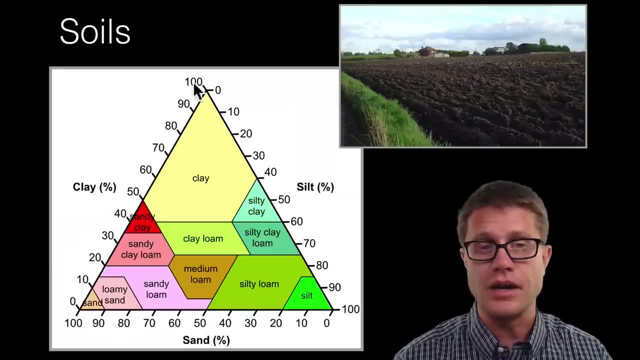 on this chart that anything that has 50% or higher clay we just call that soil clay, And we are not going to have good drainage and this is not going to be a great place to grow crops. What is the perfect soil? Well, if we have got about 20% clay and we have 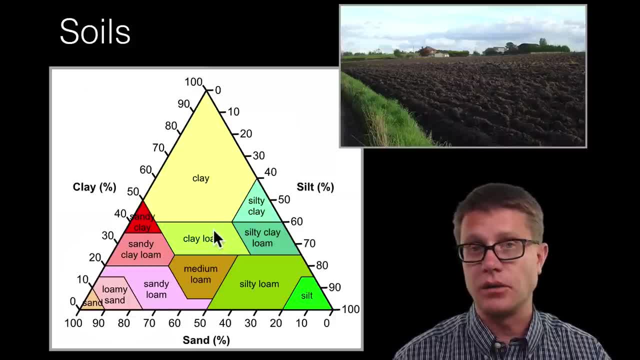 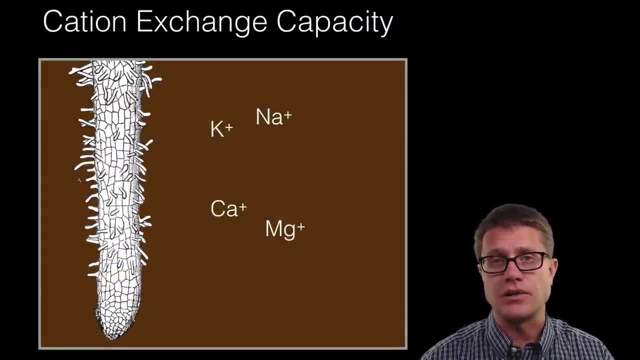 about 40% of sand and silt, we have what is called a loam And that is going to be a nice balance of all those particle sizes, Because clay is important. If we look at the cation exchange capacity, what is that? That is, the ability of a soil. 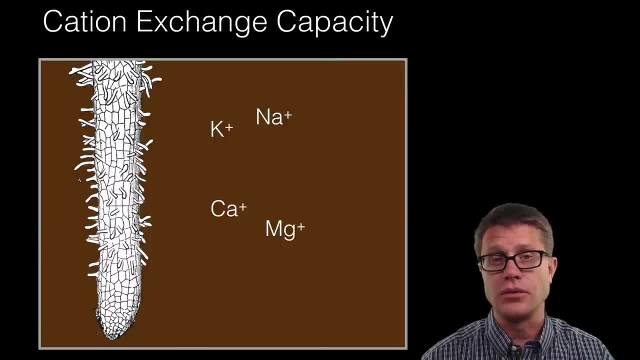 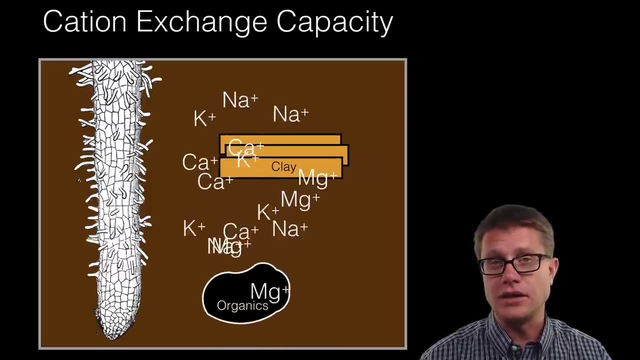 soil to deliver important ions, important nutrients, to the root itself, And the more clay we have, so this is going to be at the microscopic level- and the more organics we have, they are going to be attracting those cations and they are going to deliver it to. 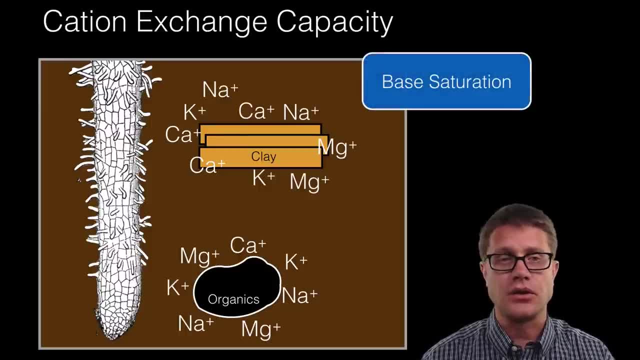 the root itself. Another important property of soil that goes along with the CEC is going to be the base saturation. So how can these minerals buffer the acidity of the soil as it comes in as well, Because that acidity can damage the plants? Soil conservation you. 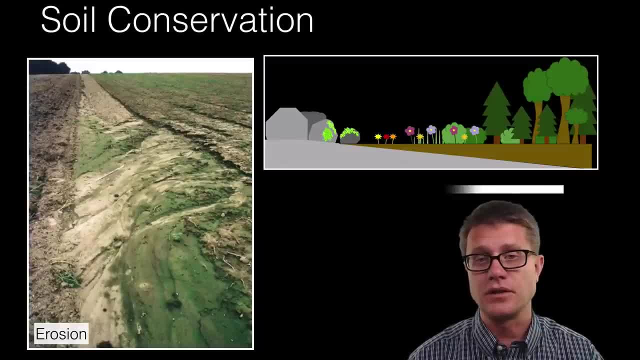 can see is incredibly important. If it takes hundreds of years to form these soils, we can turn that around overnight. So this is going to be soil erosion, where we are rinsing that top soil off, And so, as a farmer, you would want to mediate that We can also have. 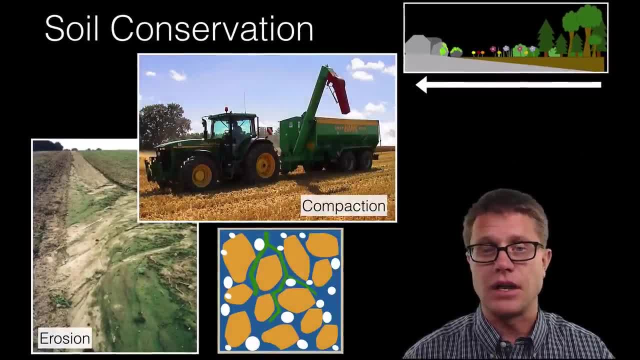 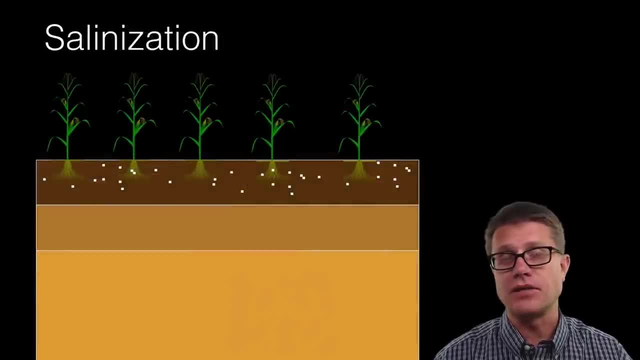 soil compaction. That is when, if the soil is wet and we are driving on it with high heavy machinery, what we can do is we can compact those pores, And so that is going to destroy that soil as well, And then we can have salinization, So increase in salt. 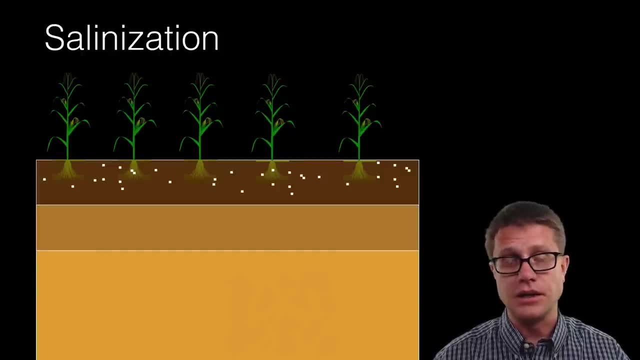 So if we have got plants growing on the soil, they are going to draw the water out And it is going to leave these natural salts behind. Normally not a problem, because we are going to have rain water. Rain water is fresh water And as we have that rain water, it pushes. 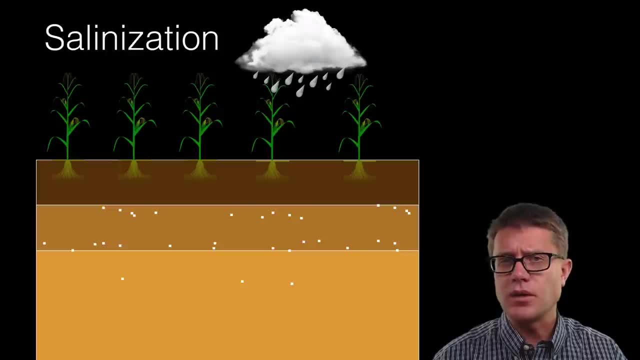 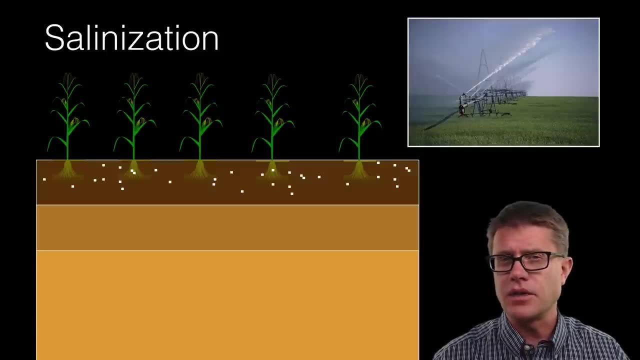 those salts out, And so it is not going to damage the crops. Now, what is the problem if we start to irrigate? So now we are going to use irrigation And we are going to spray water on the crops, Where is that water coming from? It is not coming from the sky, It is. 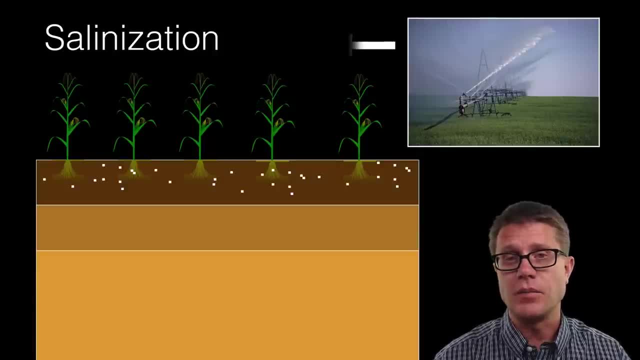 coming from the soil itself. We are probably pumping it up, And so that means that those little droplets in the irrigation are going to have salt in them, And that is going to have salts inside it, And so, as that lands on the field, we are going to increase the. 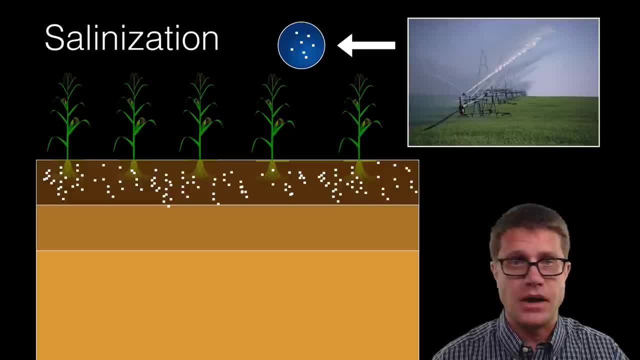 salt levels to the point where we cannot grow crops there anymore. And so how can we solve this problem? We could flush it out with fresh water. We could change the type of crops we have, Maybe get more salt tolerant crops, Or we could use crops that have bigger roots. 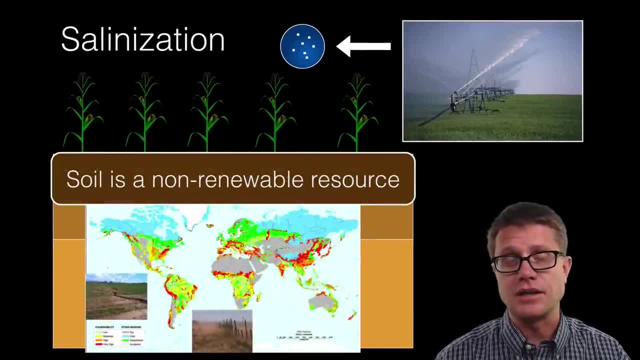 so they can push that salt farther down. But you can see what I am getting at. It is this idea that soil is a non-renewable resource. It takes a long time to form And it is really hard to balance the proper chemistry and particle size in the soil. And that is what we are. 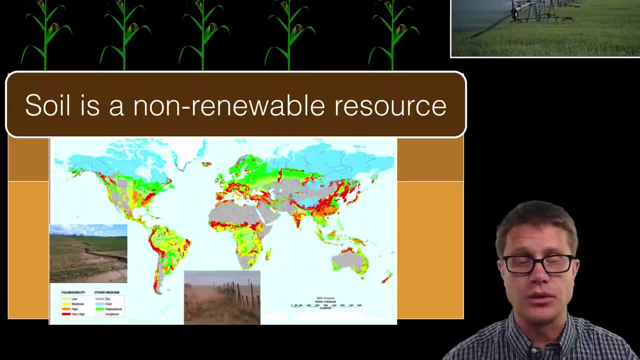 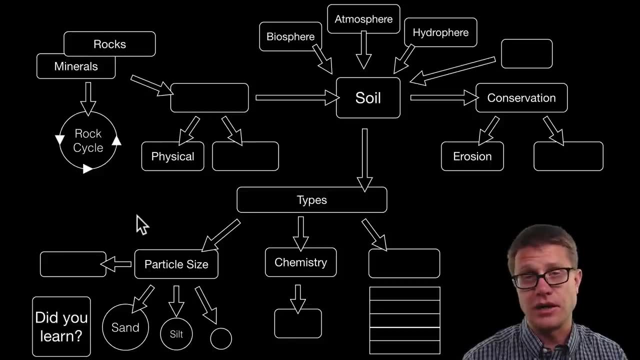 doing with soil, And this map shows us on areas on our planet where soil loss is vulnerable, And so it is important that we conserve our soil. So did you learn all of this about soils? Can you pause the video here and fill in the empty boxes? Let me show you what goes there.